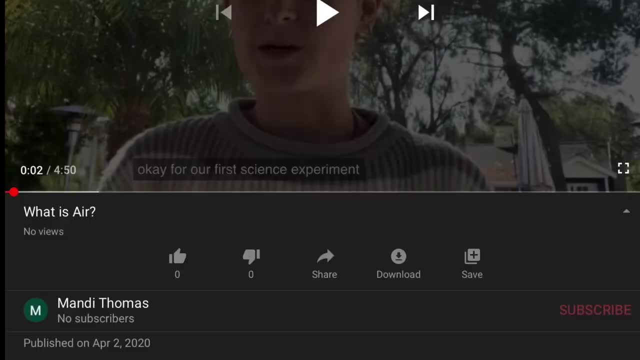 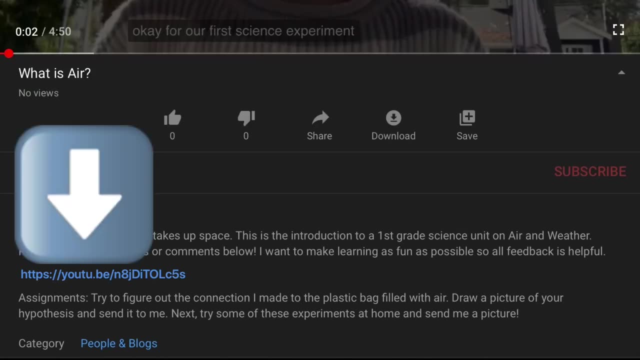 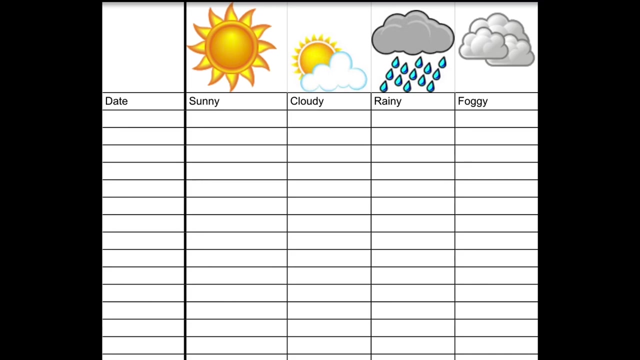 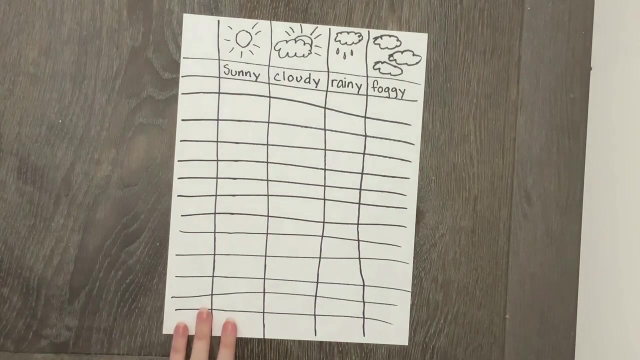 Now attached to this view. In this video below I have a link to download a better weather graph than this one, So it looks a lot better. It's easier. You don't have to draw all these lines out, So you can use that if you'd like, or use that as a model for how you want to draw your weather graph. 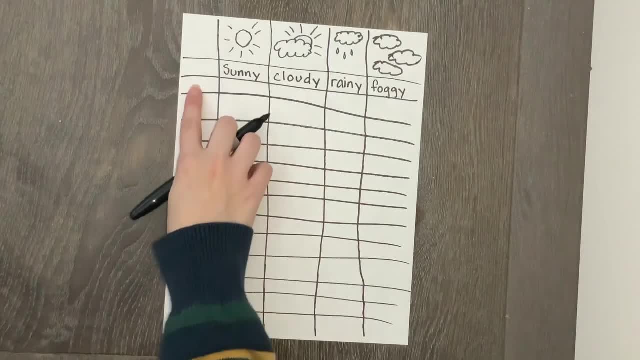 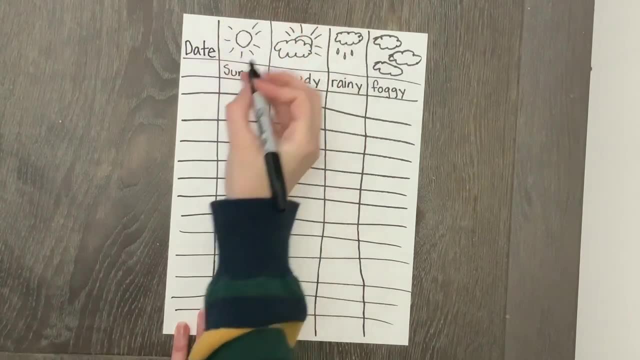 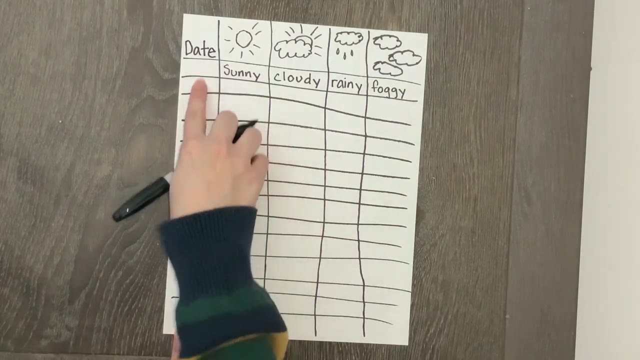 So what we're going to do down here is we're going to write our date. Remember, the E makes the A say its name, So it's D-A-T date, And then we're going to write our dates down here. We're not going to write it right here, because we have our words right here. 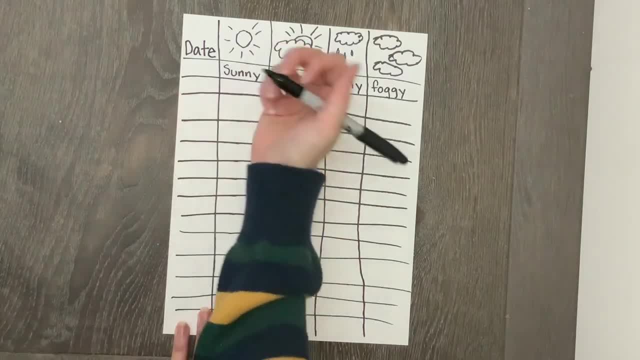 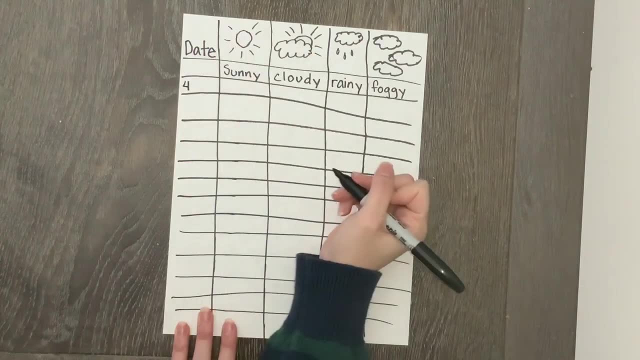 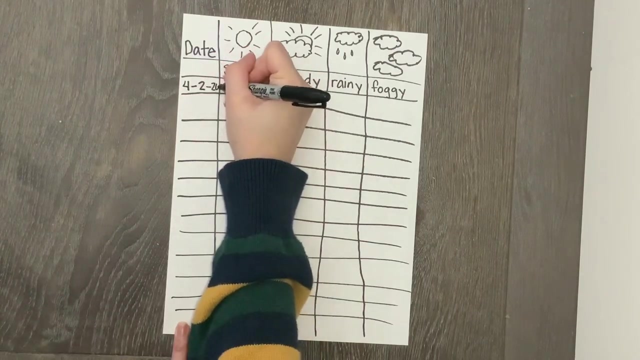 So we're going to start down here: Today is April 2nd 2020.. So I'm going to write a 4 because April is the fourth month, 2 because it's the second day, And then I'm going to write 20.. 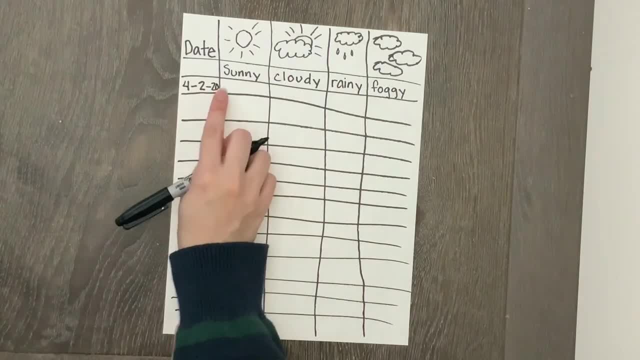 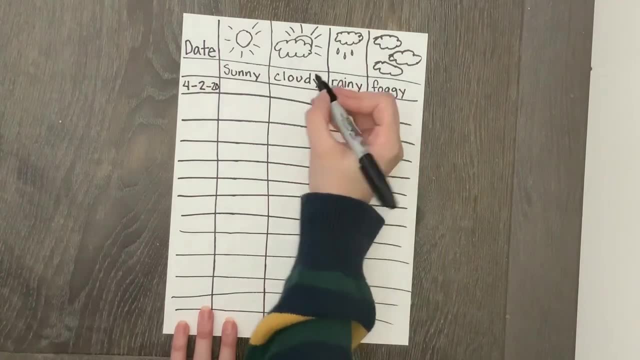 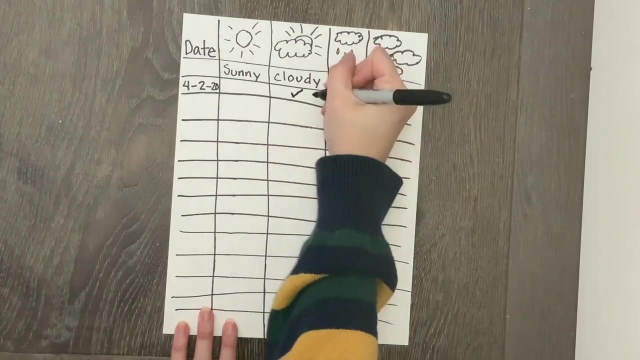 I don't really have enough space, So make sure you write with enough space. And today it's looking kind of cloudy a little bit. So I'm going to give myself a little check. A little check for today. You don't have to draw a check. You can draw a smiley face if you'd like. 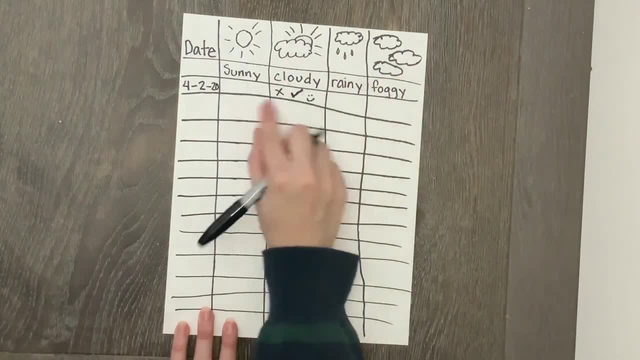 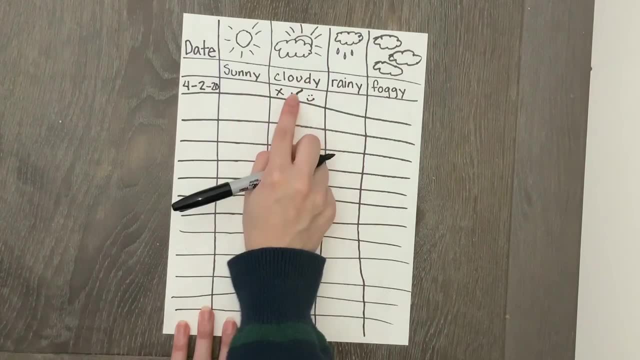 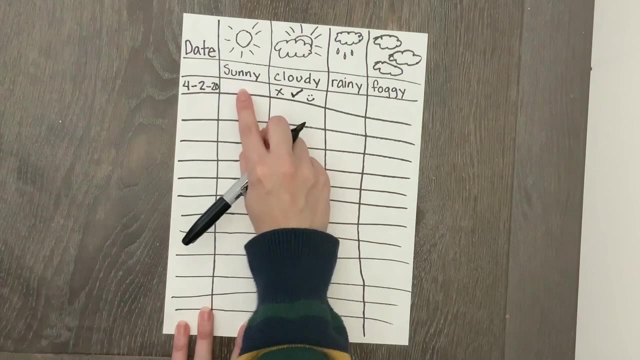 Or you can draw an X or whatever you want to draw. Maybe you want to draw an extra cloud in there. You can draw whatever you'd like, But make sure that you only do it in the one that it looks like outside. So if it looks cloudy outside, make sure you just do it in this little box and not in the sunny, rainy or foggy box. 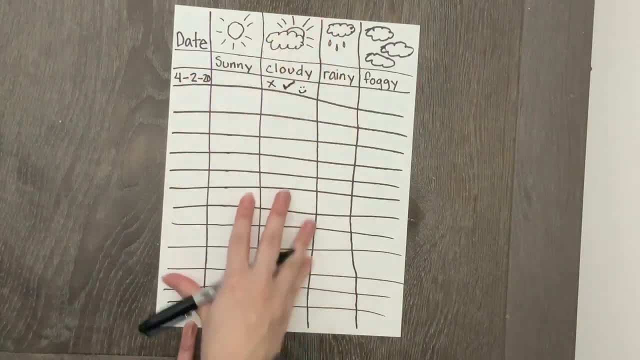 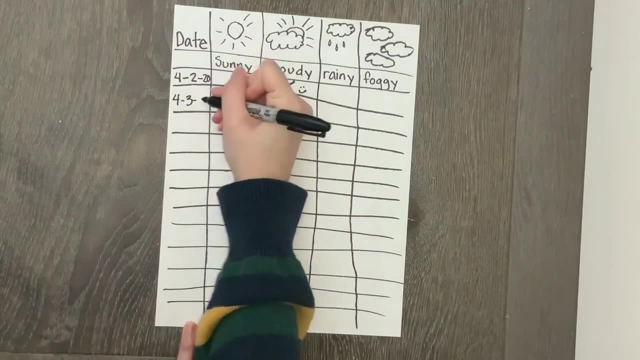 So what you're going to be doing is you're going to do this every day. So tomorrow it will be the third of April, So you're going to write 4-3-20.. And then you're going to check the day tomorrow. 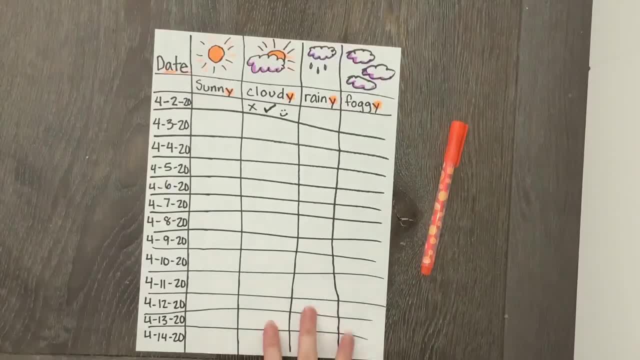 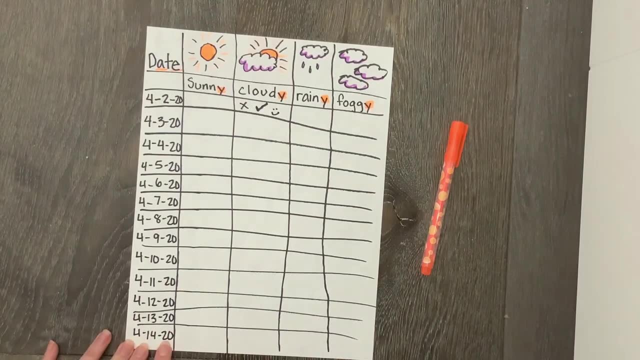 So I'm just going to finish this out really quick. So I colored this and I finished up all the dates I have until April 14, 2020.. If you have more dates, that's great. That's what I'd like. 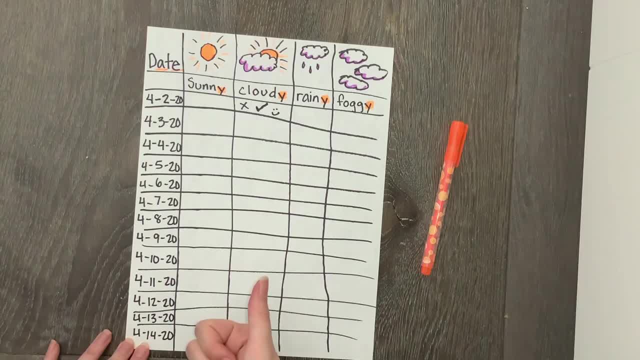 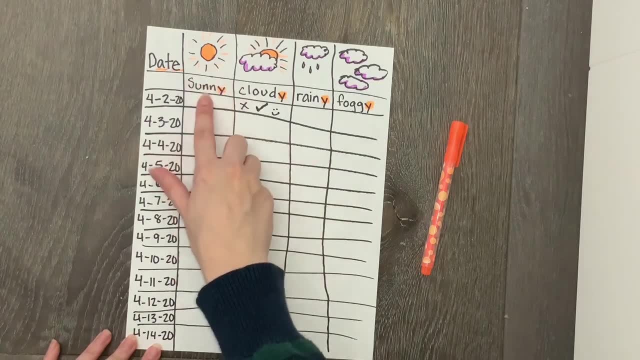 I want you to continue this as long as you can, maybe until the rest of the year, And every day we're going to look outside and see if it's sunny, cloudy, rainy or foggy. 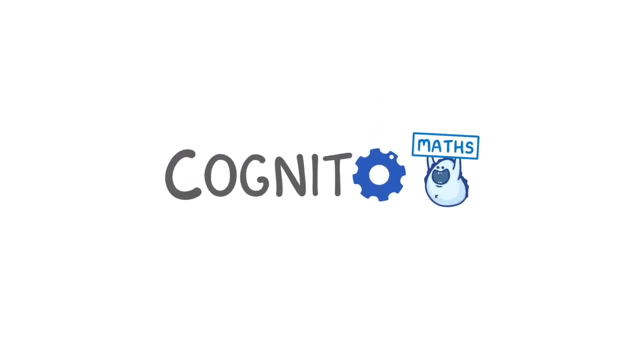 In this video we're going to look at how we can use ratios to find the coordinates of an unknown point along a line. For example, imagine that we had this graph here with a line segment between A at and B at, And then, separately, we were told that an? 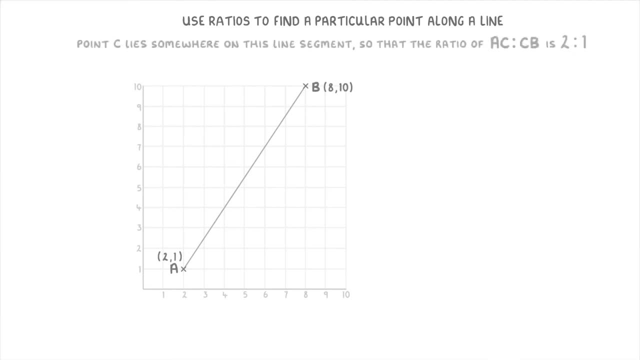 unknown point C lies somewhere along the line segment, so that the ratio of AC to CB is 2 to 1.. How would we find the coordinates of point C? Well, the first thing we need to do is think about what the ratio 2 to 1 really means. 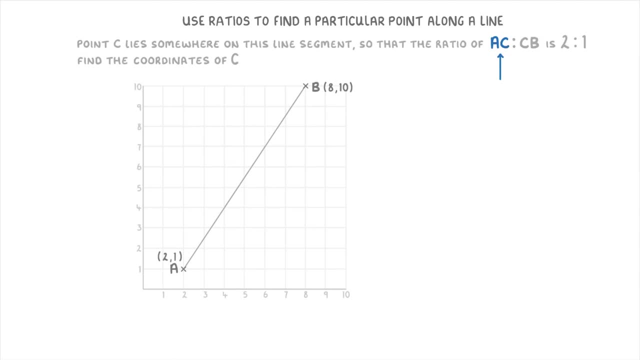 And basically it just means that the A to C section- so the distance between A and C, is 2 times B bigger than the CB section between C and B. In general, though, it's more helpful to think about it as a fraction And to convert ratios into fractions. we just take each of the numbers. 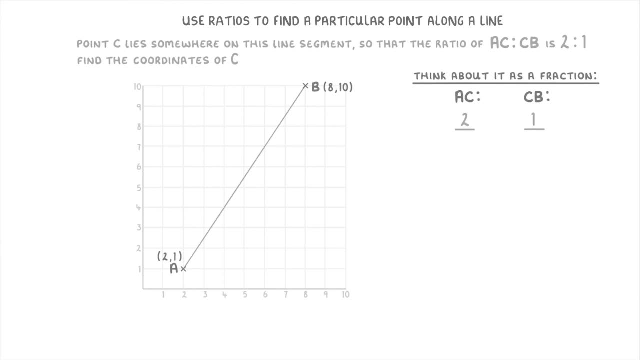 so the 2 and the 1, which become the numerators of our fractions, and then put the sum of both of them as the denominator. So because 2 plus 1 is 3, we put 3 on the bottom to give. 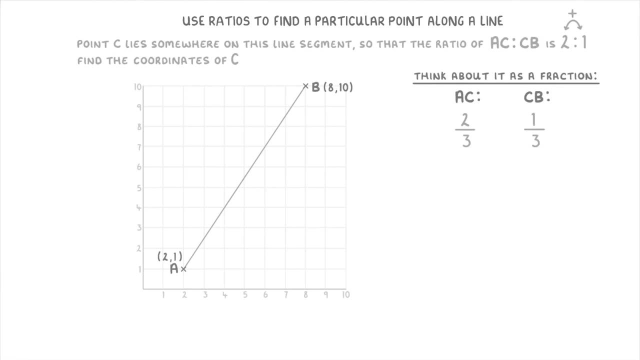 us 2 thirds and 1 third. This means that point C should be somewhere around here, so that from A to C is 2 thirds of the entire line segment and from C to B is just 1 third of the line segment. Now, I know that on this graph here we could just read off the coordinate.